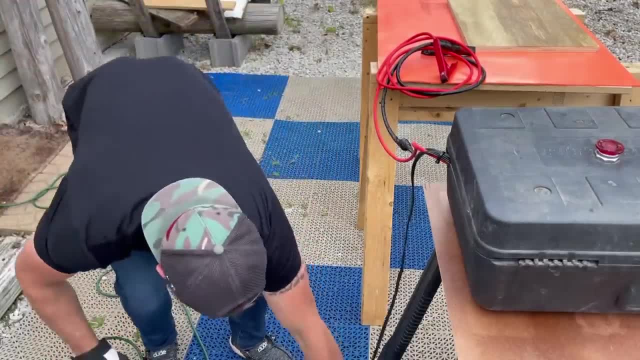 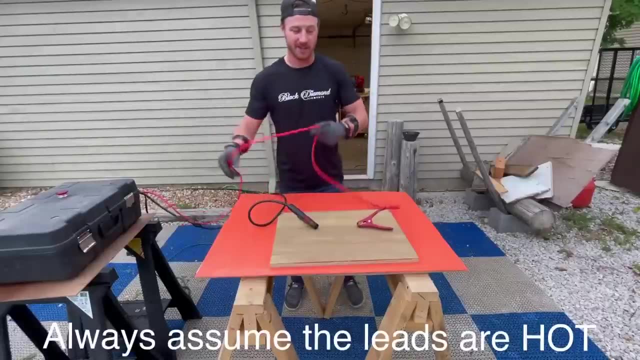 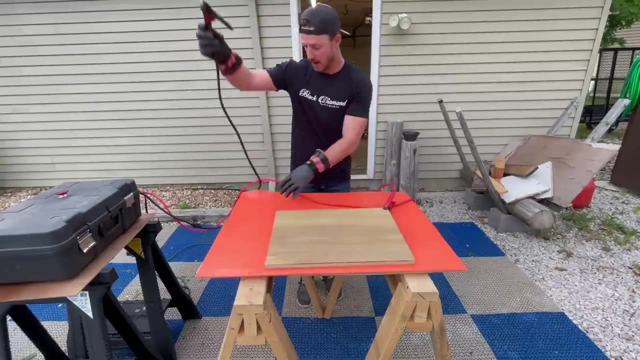 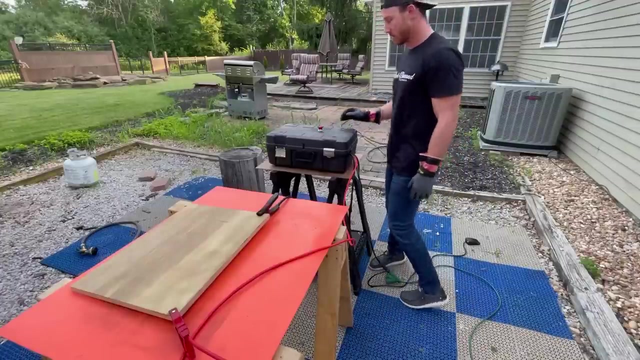 on the ground, far away from where you're working, and then you can plug this in. make sure your kill switch is off. plug that in. Anytime you're touching these cables you're going to want to have gloves on, just in case. So first you're going to want to turn on your kill switch and then you can step. 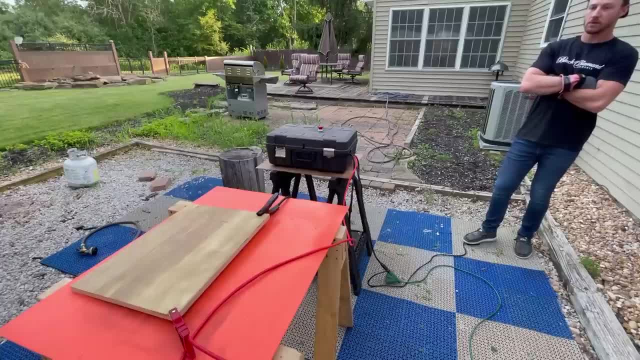 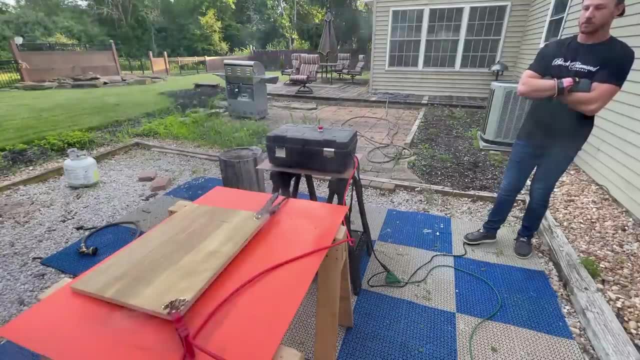 over to your dead man switch and anytime you're standing on it, the piece is going to be burning, and then anytime you step off, it's going to turn off. and I'm probably standing about five feet away from the work piece when I'm on the kill switch, so there's plenty of space between me and 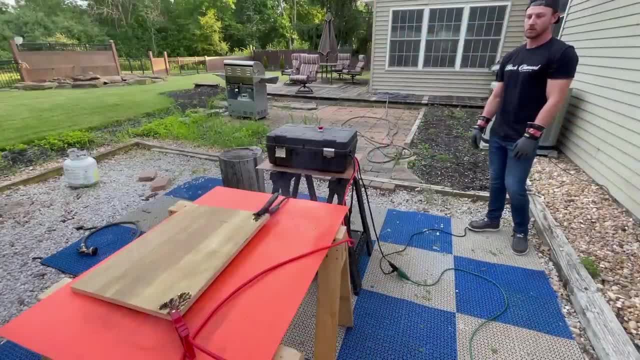 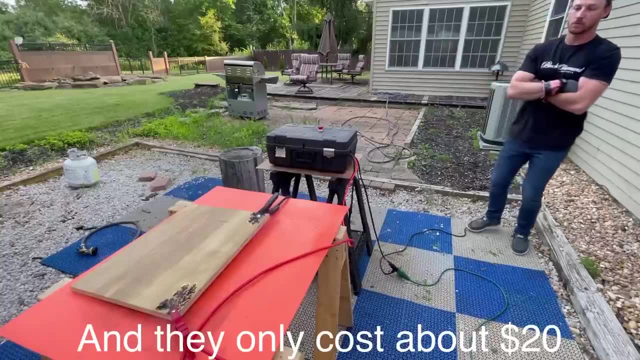 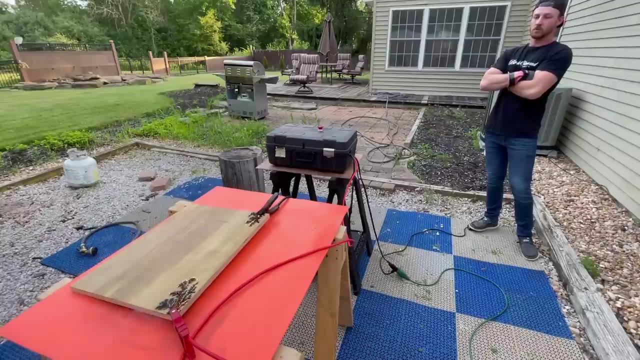 the electricity. So this dead man switch. you know they've been around forever and I don't know why I hadn't thought of using them earlier. but this thing is an absolute game changer for fractal wood burning. If the machine is only hot while you're standing on the switch, you know there's really no way you. 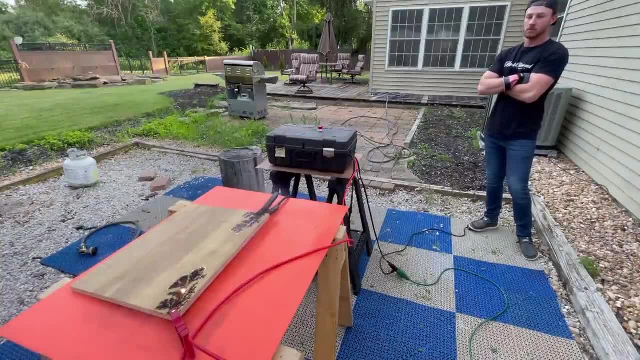 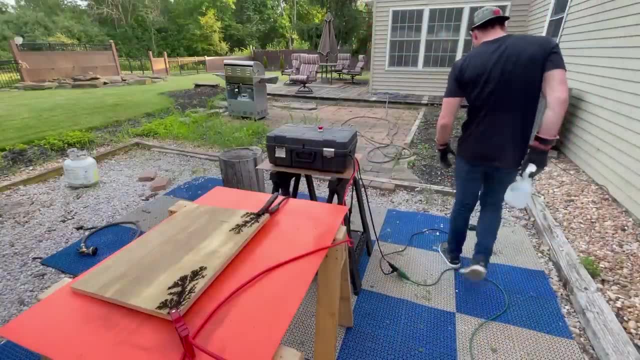 could reach over and touch it if you have the switch far enough away, and I have not. I haven't seen anyone using one of these. I found out from a guy at a local wood shop near me that's been fractal wood burning for me. 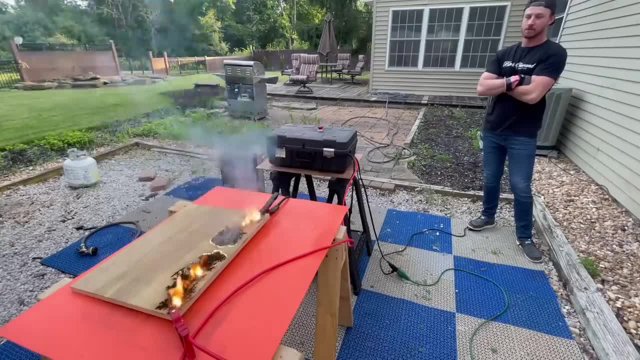 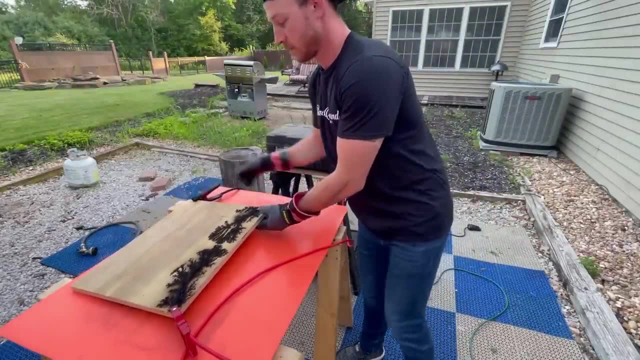 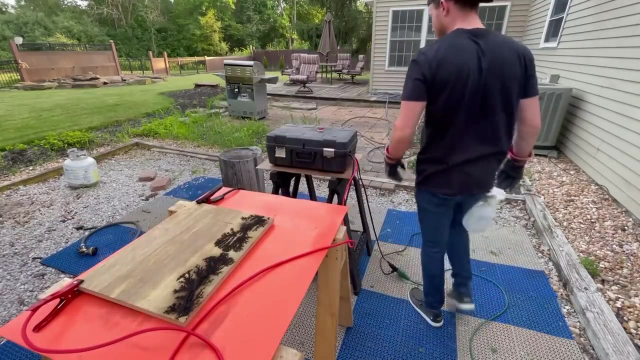 He told me about using one. so anytime you want to move these leads, you'll step off the dead man switch and turn off that kill switch before you touch the cables, and always have your rubber gloves on even if you know the machine is off. It's just a good extra precaution. so once you have the leads, 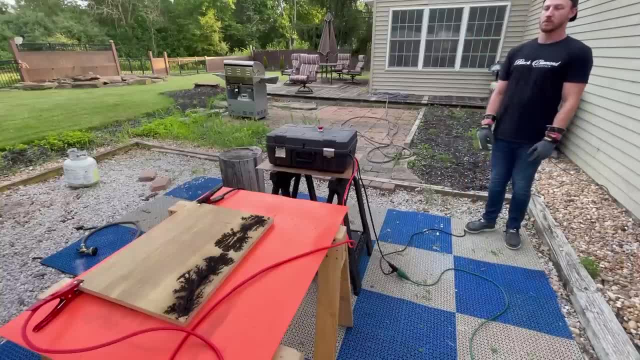 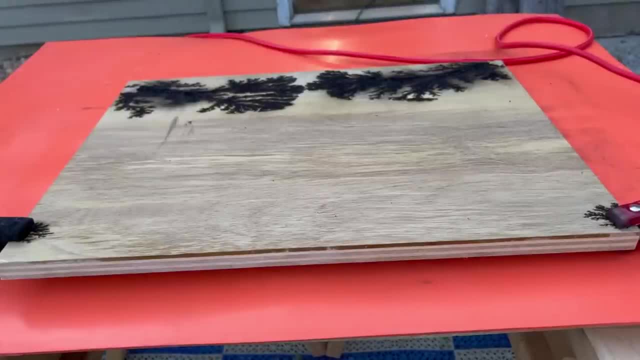 where you want them. you turn your kill switch back on and then you stand on your dead man switch and you just stay there while it's burning. I'm sure there's lots of guys out there that are using a dead man switch on their fractal wood burner and, honestly, everyone should be everyone. 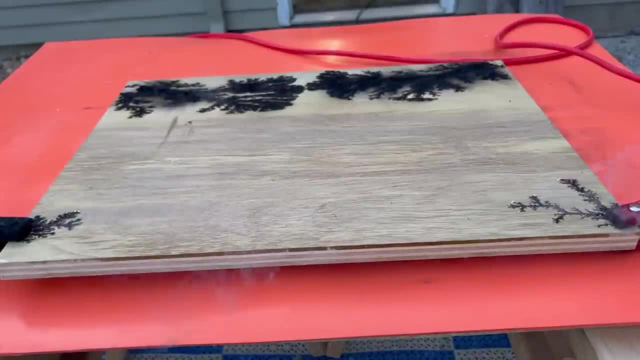 that's doing fractal wood burning should absolutely have one of these. it's just a much safer way to do this. you know, like I said, if you set it up far enough away to where, if you're standing on it, you can't possibly touch the workpiece, you're going to be much, much safer, and I will add the.